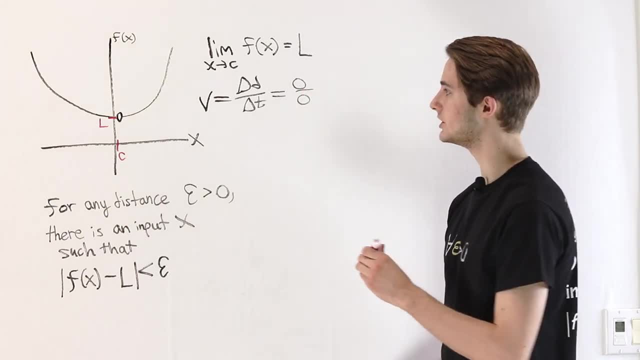 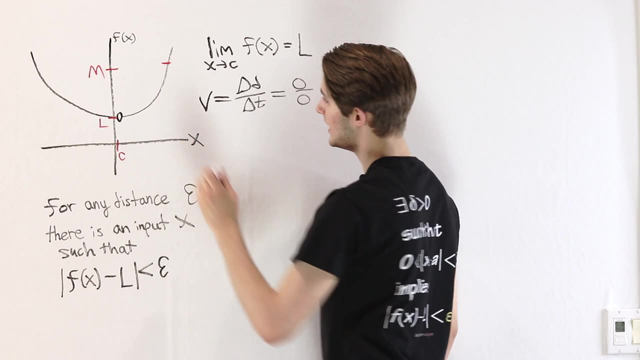 work. Well, there's one problem. Let's say, instead of trying to prove that the limit was l, we wanted to prove that it was some other value, m, For any distance epsilon greater than zero from that output m. there's going to be an input in here that gives us a distance less than 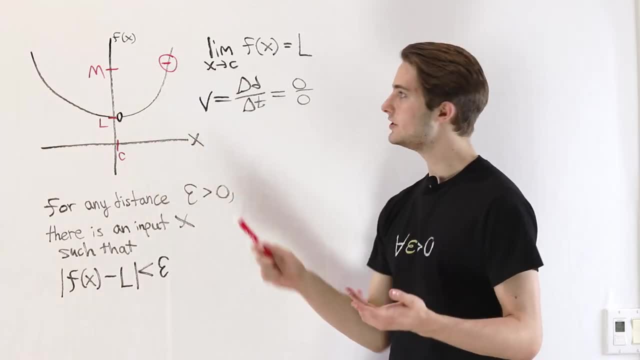 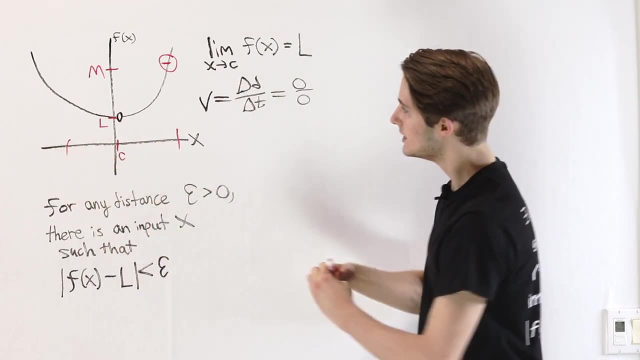 epsilon. but that's not our limiting value at c, because because input values near m are very far away from c and if we think about the range of values within that distance of c, there's a huge variance in the vertical values. To solve this, maybe, instead of thinking about specific inputs. 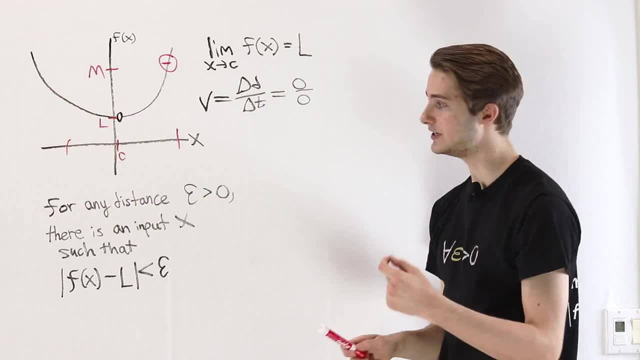 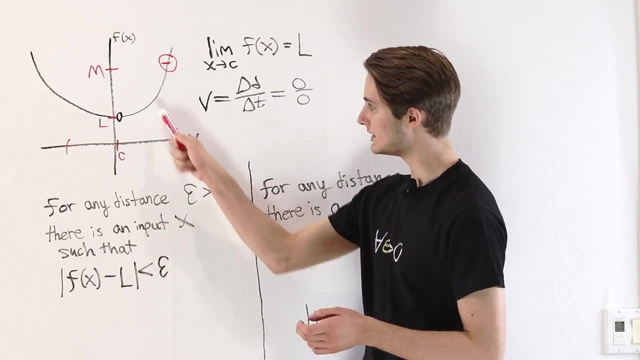 we think about ranges and then we can center those ranges of inputs around c so that our limit is specific to that input value. Before we said for any epsilon we could find a point where the distance from l was less than or equal to the input value c. Then we can calculate the value of the input values. 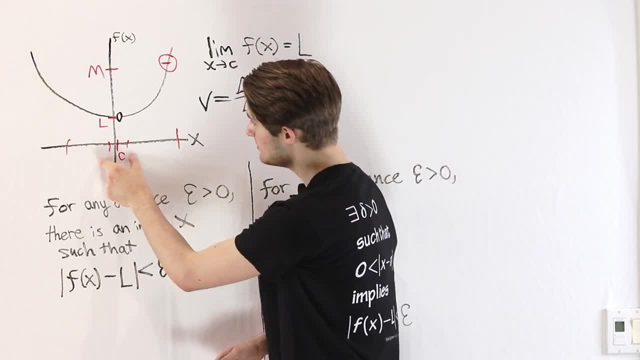 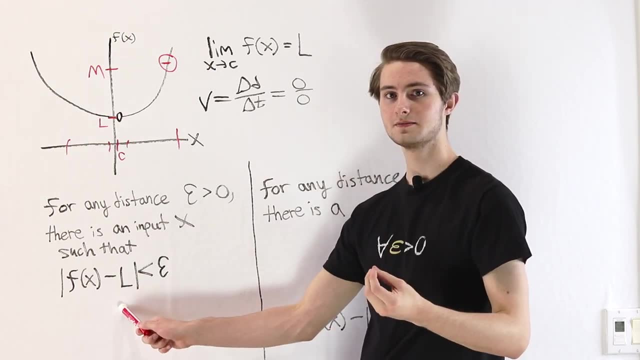 L is less than epsilon. But if we examine our function around the input C, we see that every output within a certain distance of C is also within a certain distance of L. On the other hand, no range centered at C will have every output close to M, because 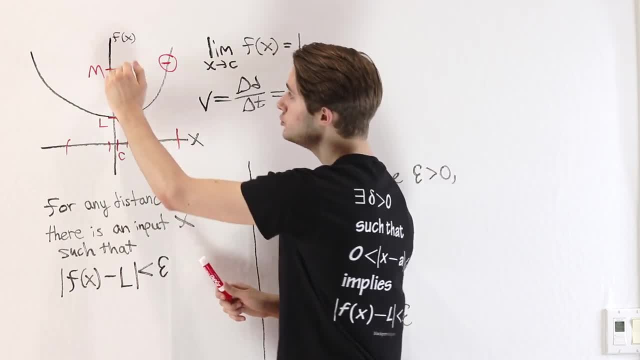 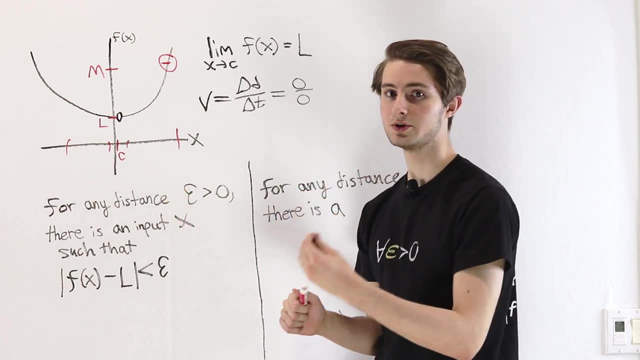 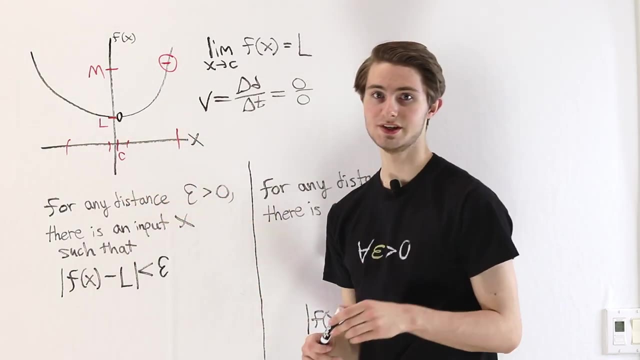 we'll always have these values down here next to C that are super far away from M. So if we choose an epsilon smaller than that distance, there's no range centered at C where every output is within a distance epsilon of M. Now we have to define our idea of a range. Remember that the range is centered around. 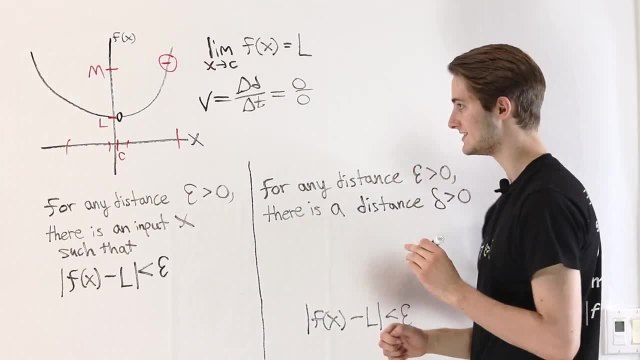 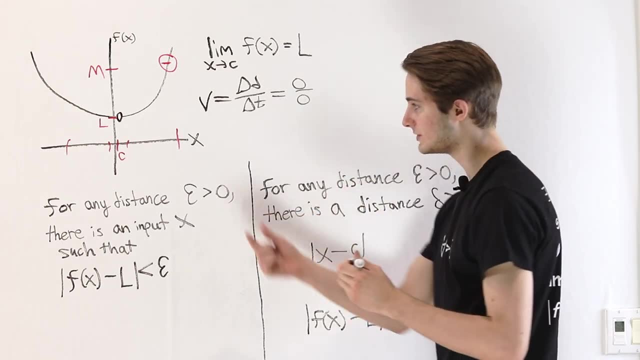 C. so we can define it simply in terms of some positive distance, delta away from C. If we want every value in that distance, we can just say that the magnitude of the difference between our input X and C must be less than delta. We'll also say that the distance 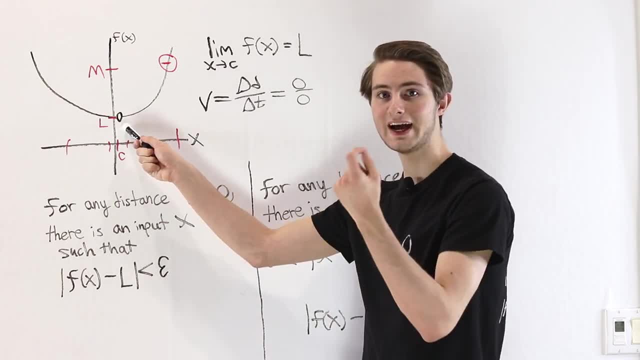 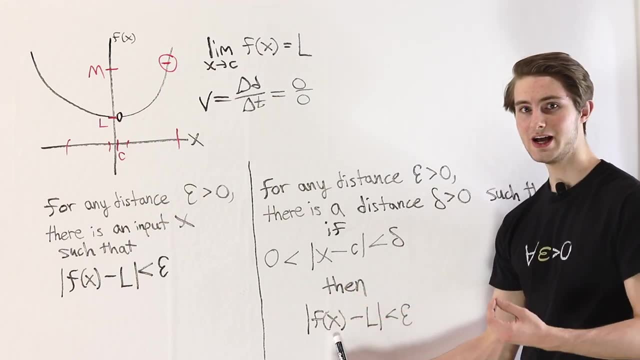 is greater than zero. to avoid the problem of the hole at the actual value of C, We saw that if our input X is within that distance delta from C, then the output of output f of x must be within epsilon of L. So this is the formal epsilon delta definition. 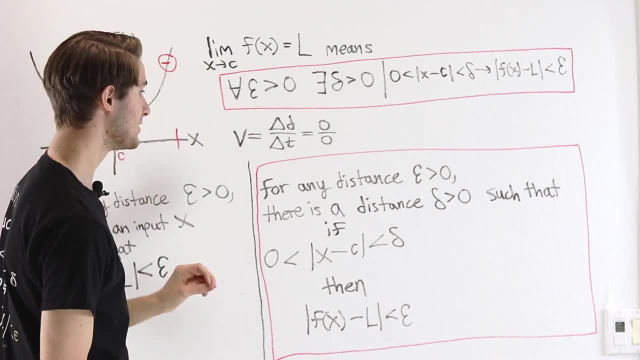 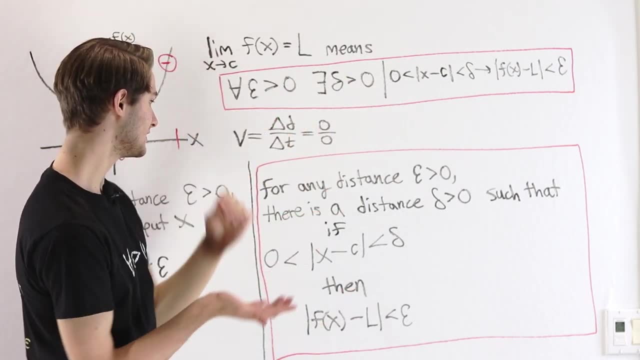 of a limit, and I've also written the same thing in more technical notation up here, Because limits are about functions approaching a particular input. we say that for any distance around that limiting value L, we can find a range where every value in that range is.